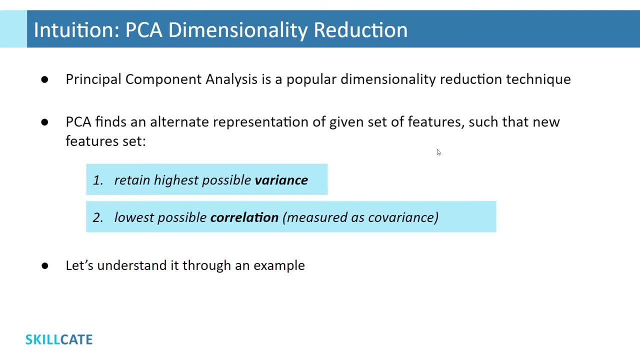 It uses a mathematical approach to find an alternate representation of the given feature set, ensuring retention of highest possible variance and minimization of correlation among features. Let's understand these two points further with the help of an example. Firstly, let's discuss how PCA retains the highest possible variance. 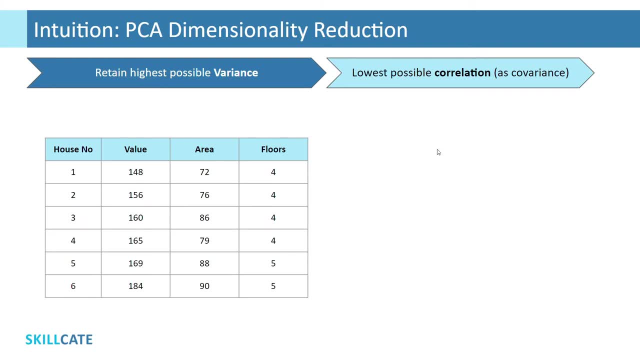 Over here. we have data of six houses capturing three features: Value of the house, total area and number of floors. Let's analyze this data from a PCA dimensionality reduction standpoint and understand which variables are more important than others. For this we would need variances for these individual features. 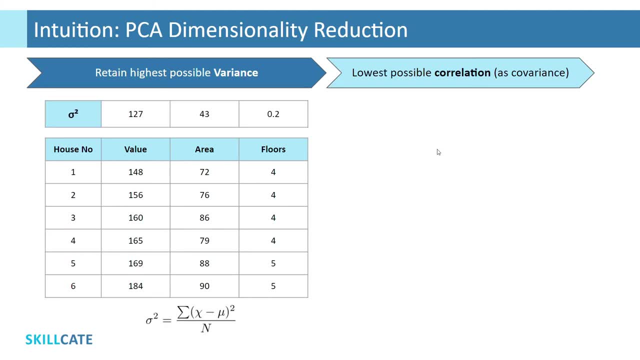 We have already done this computation For your reference. this is the formula for variance. With this information, we can clearly observe that floor has a very small variance value. From an intuition standpoint, what this means is that I cannot distinguish one house from another using this feature. 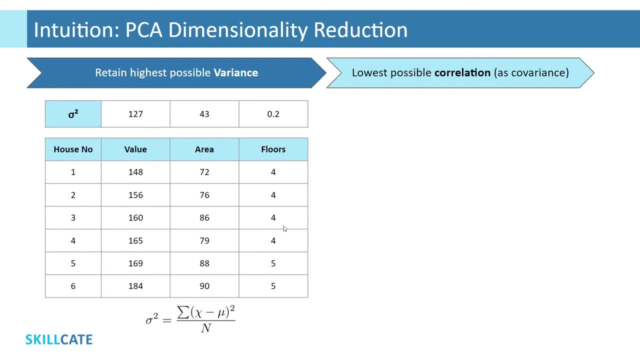 As you may see, floors are almost similar for all six houses and certainly do not help us much in distinguishing one house from another. Now, if we plot number of floors with house value on this two-dimensional chart, we may observe very small variation along y-axis, which is floor. 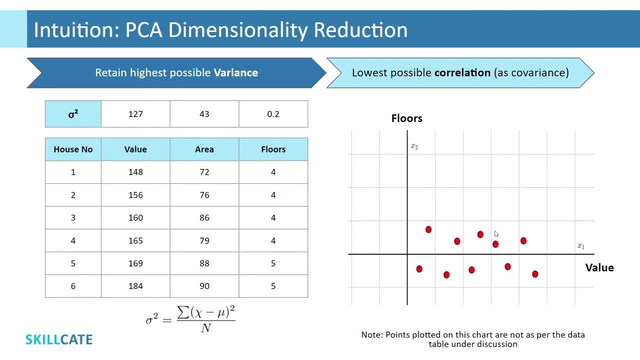 when x-axis, which is value, shows a lot of variation. Value, by the way, has a contrastingly high variance anyway, And at this point it would make a lot of sense if we could reduce this two-dimensional chart to a single dimension. 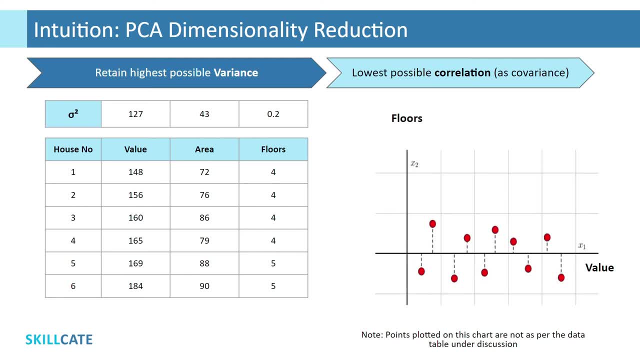 For that, we would project these red points to x-axis, which is value of the house, and voila, We have successfully dropped one variable. As you may observe, we still are able to retain almost the entire variance through these two variables that are contributing the majority of it.